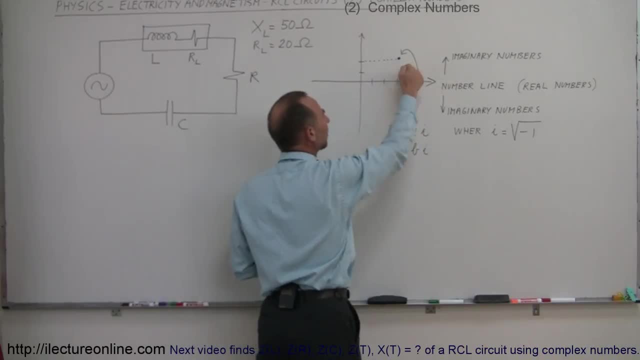 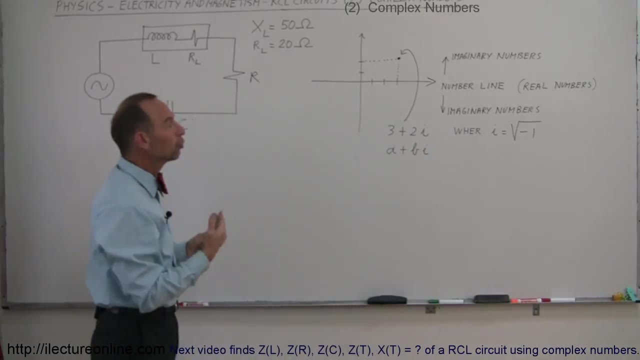 So we can write this as 3 plus 2i. that would be this number right there off the number line, two units away from the number line. so the imaginary part has a magnitude or an amplitude of two units. So let's now see how we can relate that to our RCL circuit. 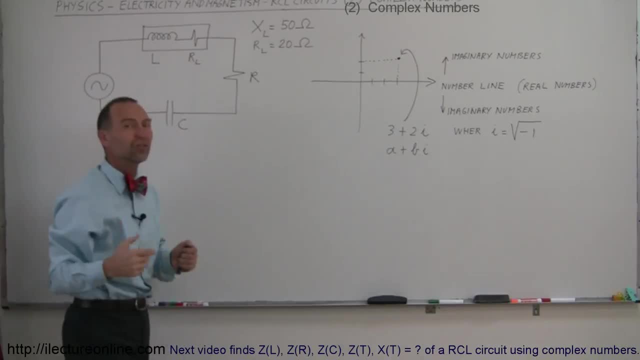 Now here we have an inductor. Usually inductors have a small amount of resistance to them because an inductor is a small amount of resistance to an inductor. There's a long wire that's coiled up, and a long piece of wire does have some resistance. 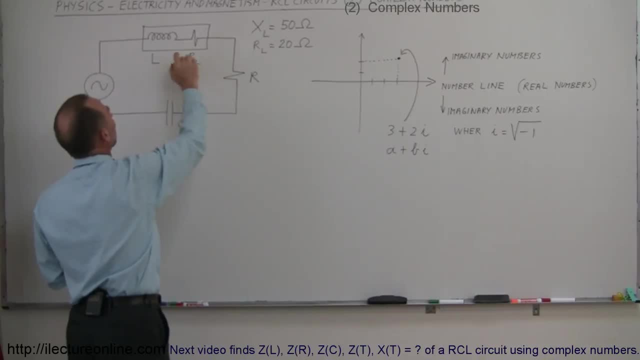 So let's call that Rcibel for the resistance of the inductor, and of course then we have the inductor part as well. We still have a resistor here, we still have a capacitor, but let's only concentrate on the inductor. 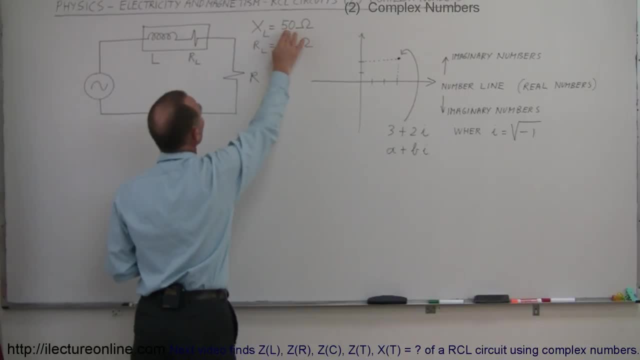 In this case, the opposition to the current of the inductor is 50 ohms, and then the resistance of the inductor, Rcibel, is 20 ohms. Now we don't really talk about resistance of an inductor. we tend to talk about it in terms of reactants. 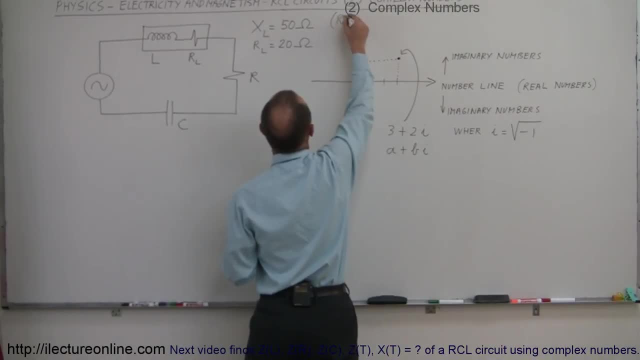 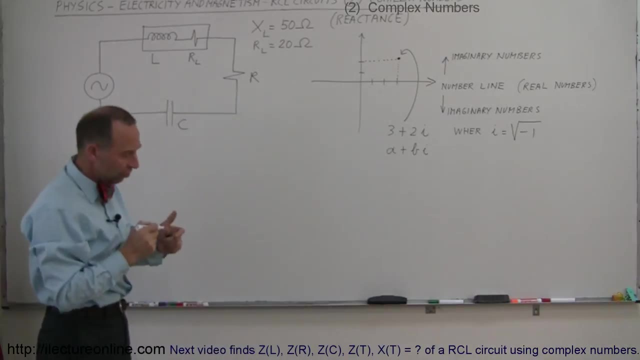 So we call the X as we call it, we use the letter X, we call that reactants and it's something like resistance. it has the same units as resistance, but the reason why we call it reactants is because it reacts to the time-varying voltage from the source. 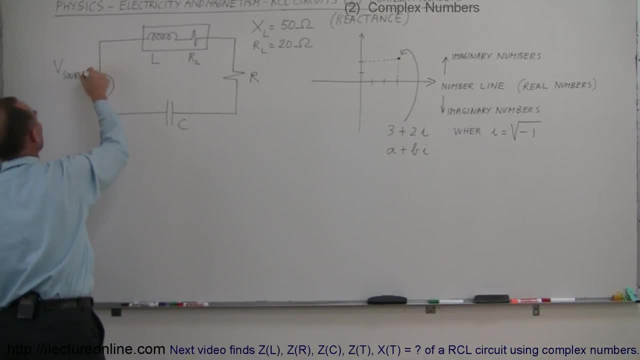 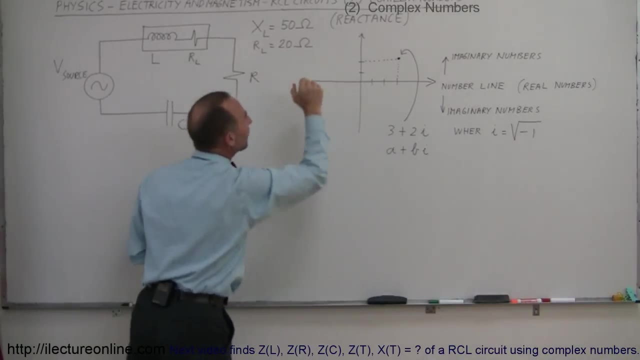 So this is the voltage from the source and as the source changes over time, because it oscillates between max and min, then it reacts to that changing voltage source. therefore we call it reactants, but it's kind of like resistance. So think of reactants, kind of like resistance. 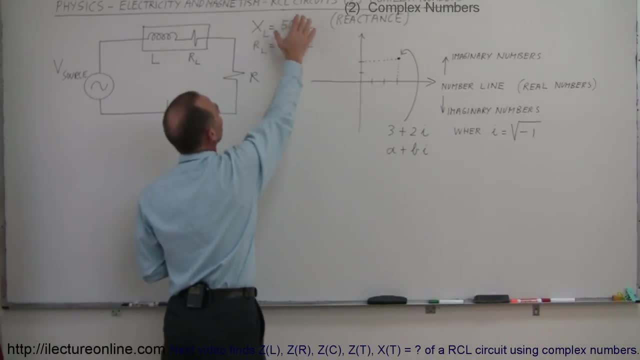 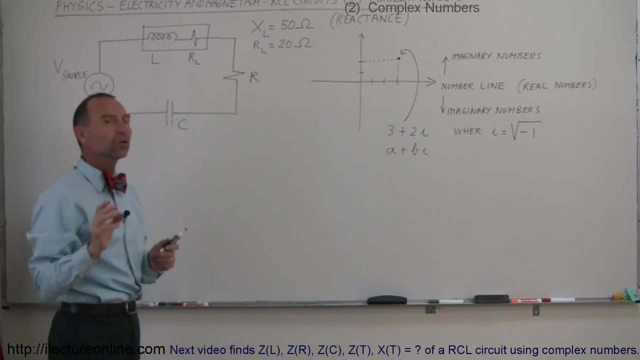 But reactants, is considered the imaginary part of the total opposition to the current. So we're going to write the total opposition to the current in terms of a complex number and we're going to call it impedance. So Z, which is a term, again it's another term, it's again opposition to current. 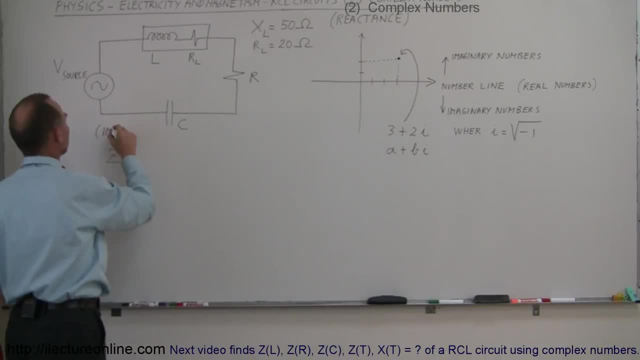 but it's a combination of the real and imaginary part together. So the impedance of a component against the current flux is equal to the real part of the impedance, which is the resistance, plus the imaginary part of the opposition, which is the reactants. 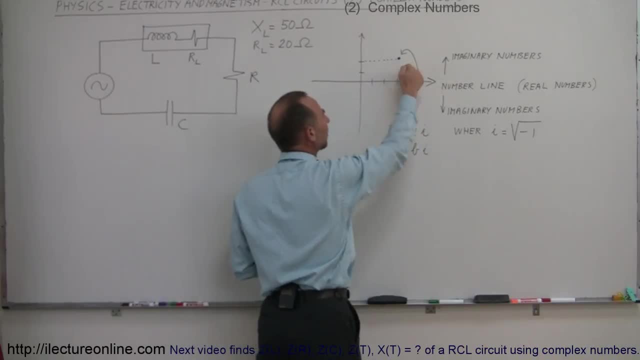 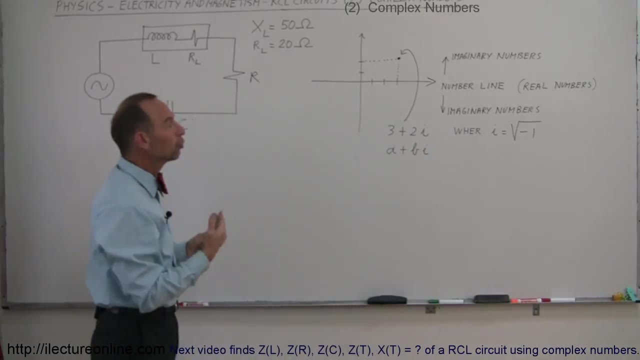 So we can write this as 3 plus 2i. that would be this number right there off the number line, two units away from the number line. so the imaginary part has a magnitude or an amplitude of two units. So let's now see how we can relate that to our RCL circuit. 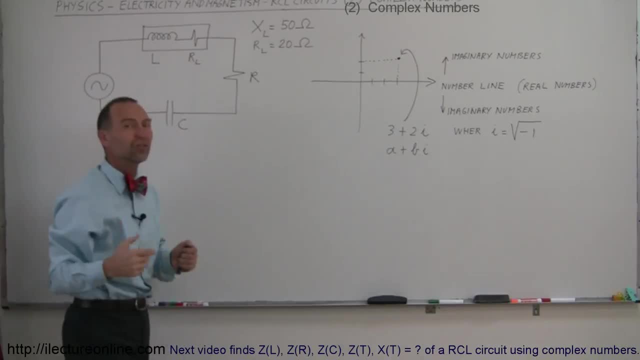 Now here we have an inductor. Usually inductors have a small amount of resistance to them because an inductor is a small amount of resistance to an inductor. There's a long wire that's coiled up, and a long piece of wire does have some resistance. 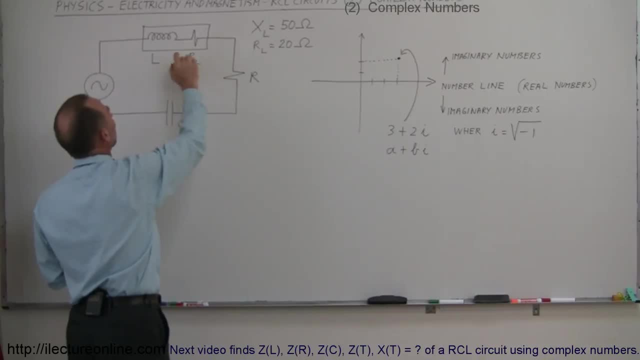 So let's call that Rcibel for the resistance of the inductor, and of course then we have the inductor part as well. We still have a resistor here, we still have a capacitor, but let's only concentrate on the inductor. 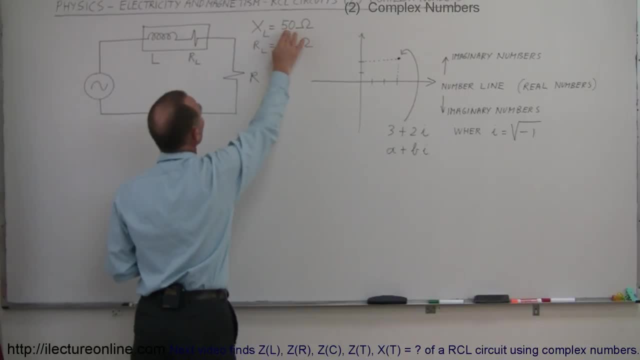 In this case, the opposition to the current of the inductor is 50 ohms, and then the resistance of the inductor, Rcibel, is 20 ohms. Now we don't really talk about resistance of an inductor. we tend to talk about it in terms of reactants. 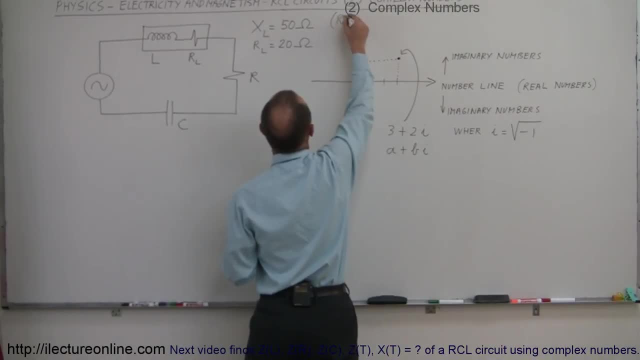 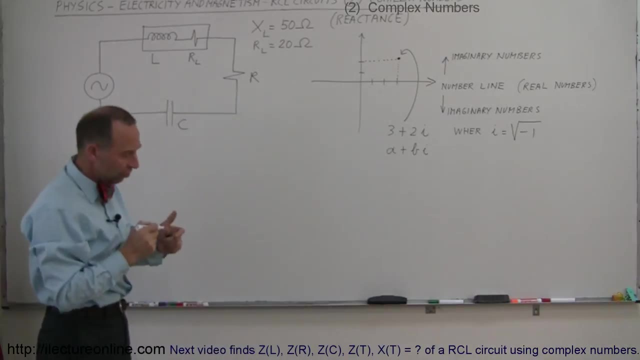 So we call the X as we call it, we use the letter X, we call that reactants and it's something like resistance. it has the same units as resistance, but the reason why we call it reactants is because it reacts to the time-varying voltage from the source. 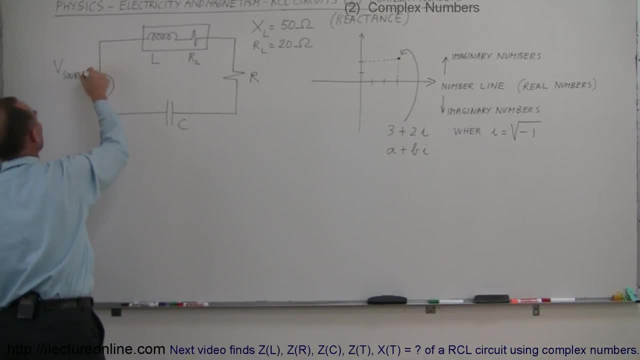 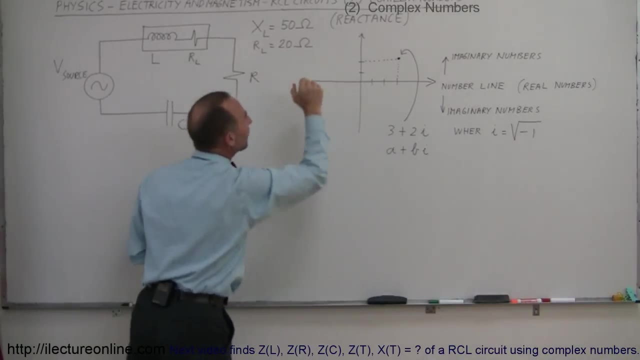 So this is the voltage from the source and as the source changes over time, because it oscillates between max and min, then it reacts to that changing voltage source. therefore we call it reactants, but it's kind of like resistance. So think of reactants, kind of like resistance. 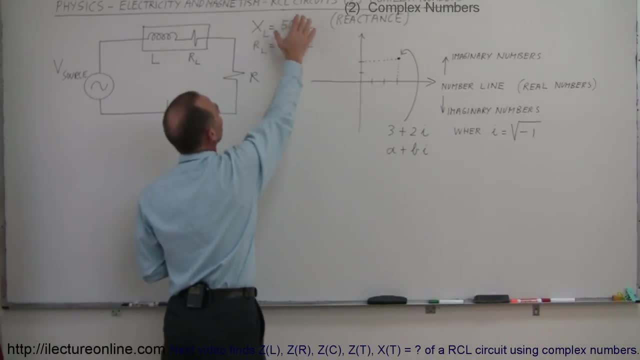 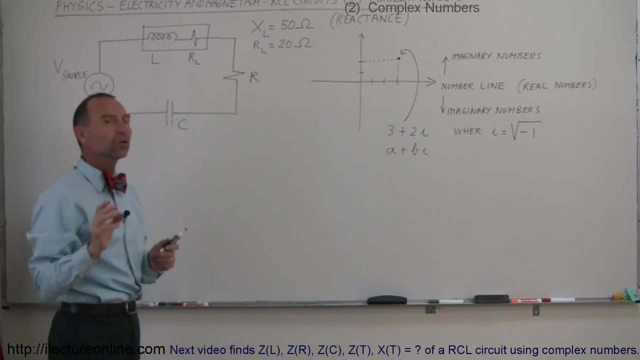 But reactants, is considered the imaginary part of the total opposition to the current. So we're going to write the total opposition to the current in terms of a complex number and we're going to call it impedance. So Z, which is a term, again it's another term, it's again opposition to current. 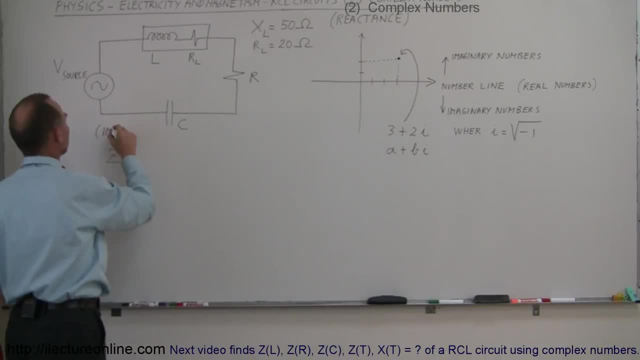 but it's a combination of the real and imaginary part together. So the impedance of a component against the current flux is equal to the real part of the impedance, which is the resistance, plus the imaginary part of the opposition, which is the reactants. 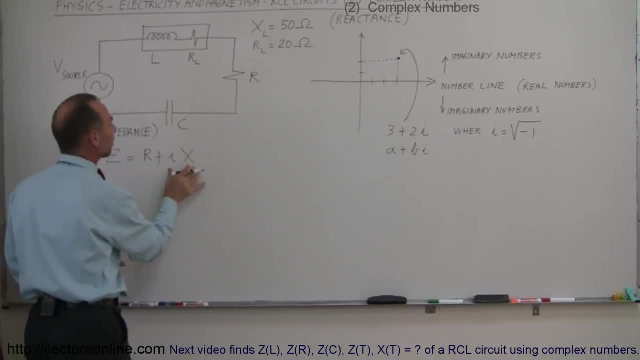 So the impedance is the sum of the real part and the imaginary part. again, I is the square root of negative 1, and so again, it's one of those complex numbers. So in the case of this particular inductor we can say that the impedance of the inductor is equal to the resistance of the inductor. 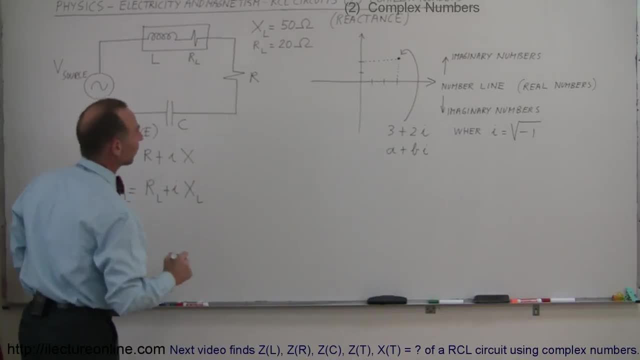 plus I times the reactants of the inductor and we call that resistance. So in this case we can see that Z sub L is equal to 20 ohms. that's the real part of the opposition which came from the resistor in the inductor. 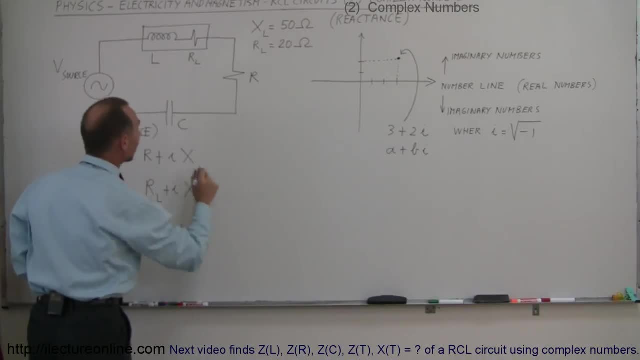 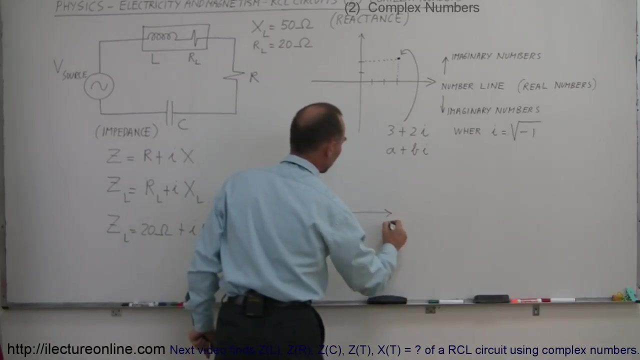 the resistive property of the inductor plus I times 50 ohms, And that would be the impedance of that inductor. Now if we're going to draw that on a graph, it would look like this: Notice: the horizontal axis would indicate the resistance. 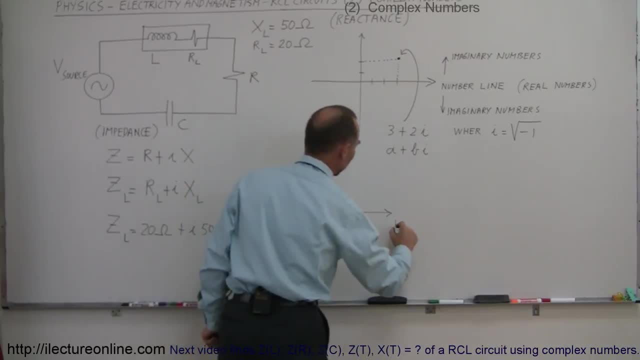 the vertical axis would indicate the reactants. so this is X, this is R. Notice it's 20 ohms of the real part. so let's say that's 10, 20 ohms. right there, 20 ohms. 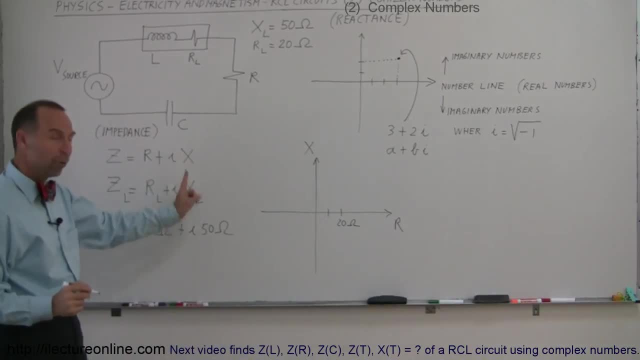 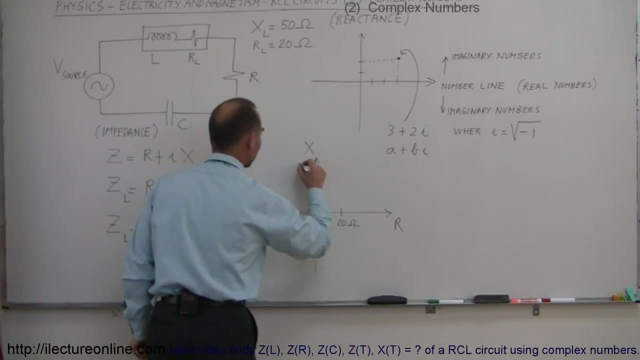 and then we have 50 ohms in the positive Y direction, so to speak, or the positive reactants direction. so that's 10,, 20,, 30,, 40,, 50, there we go. And then, when we combine these two together, 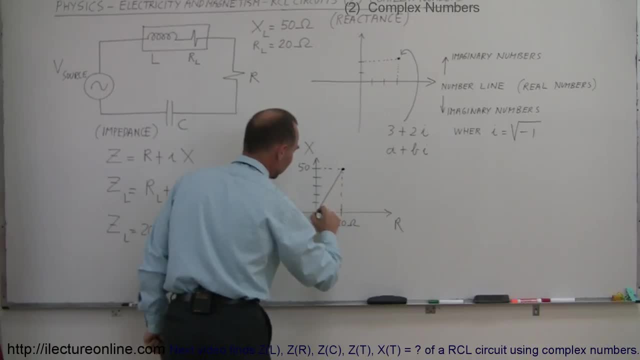 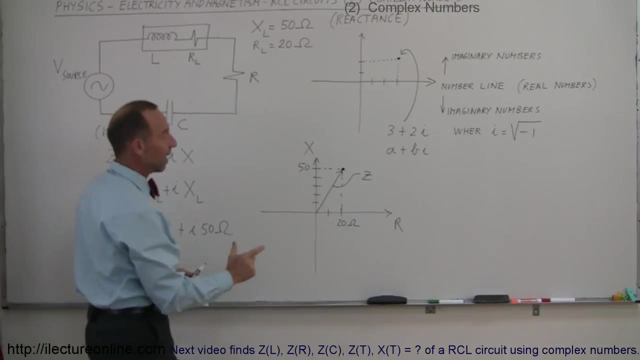 there, they meet right there, and this here is what we would call the impedance, That's, the impedance of that particular component, and that impedance has a real part caused by the resistance, and an imaginary part caused by the coil or the inductor. 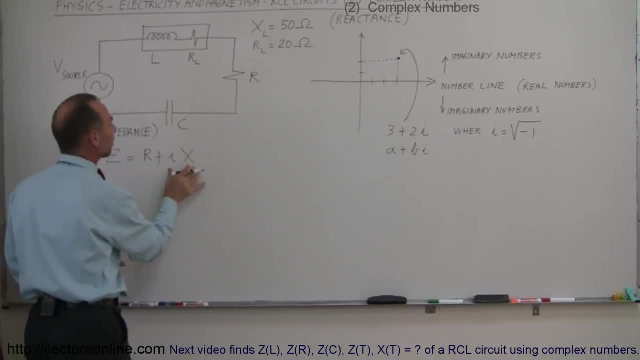 So the impedance is the sum of the real part and the imaginary part. again, I is the square root of negative 1, and so again, it's one of those complex numbers. So in the case of this particular inductor we can say that the impedance of the inductor is equal to the resistance of the inductor. 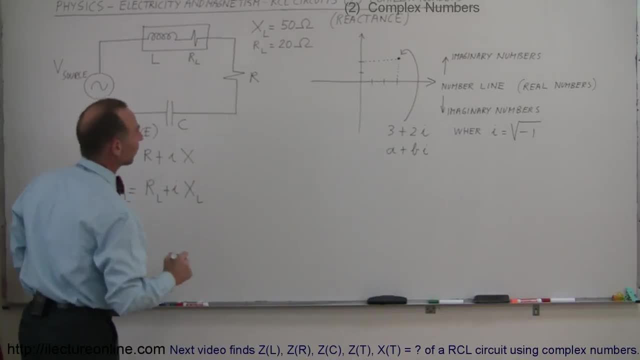 plus I times the reactants of the inductor and we call that resistance. So in this case we can see that Z sub L is equal to 20 ohms. that's the real part of the opposition which came from the resistor in the inductor. 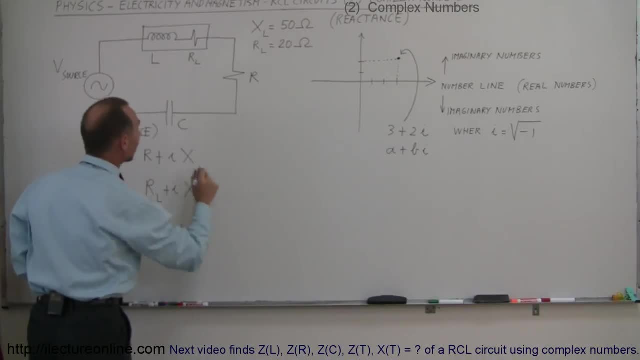 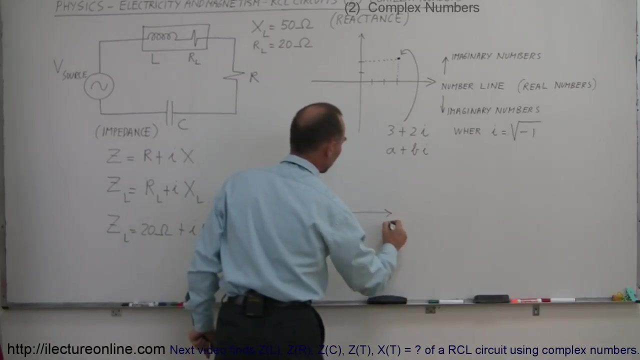 the resistive property of the inductor plus I times 50 ohms, And that would be the impedance of that inductor. Now if we're going to draw that on a graph, it would look like this: Notice: the horizontal axis would indicate the resistance. 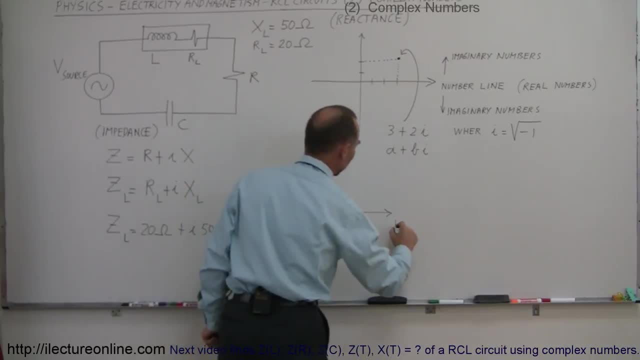 the vertical axis would indicate the reactants. so this is X, this is R. Notice it's 20 ohms of the real part. so let's say that's 10, 20 ohms. right there, 20 ohms. 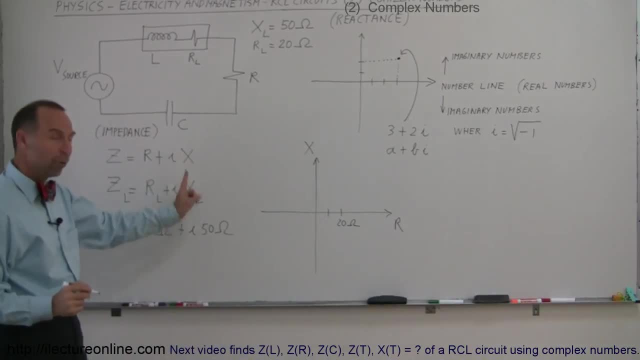 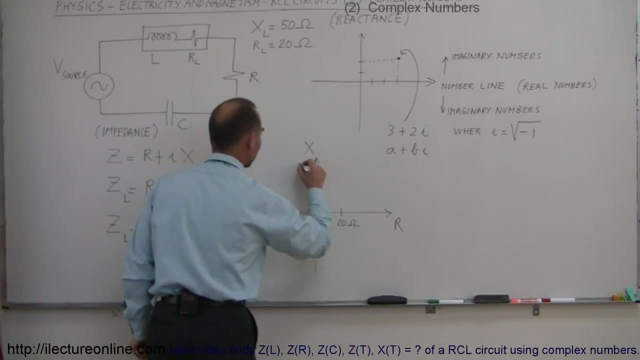 and then we have 50 ohms in the positive Y direction, so to speak, or the positive reactants direction. so that's 10,, 20,, 30,, 40,, 50, there we go. And then, when we combine these two together, 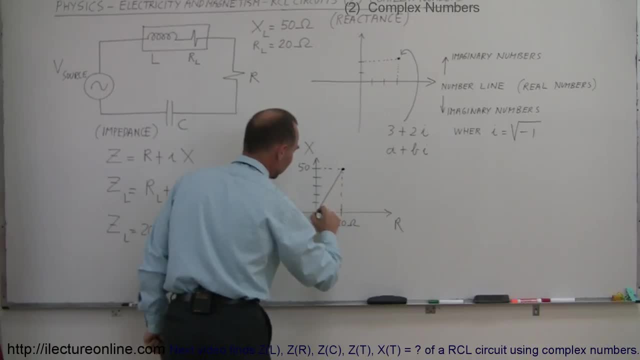 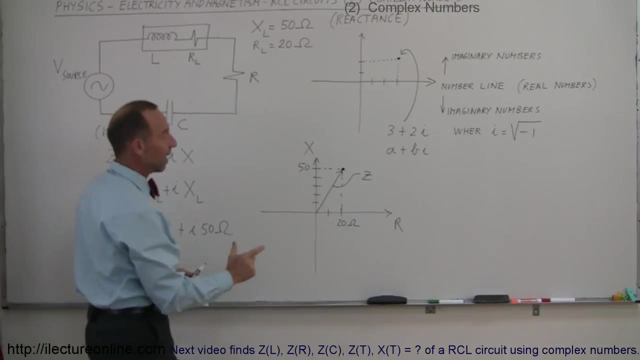 there, they meet right there, and this here is what we would call the impedance, That's, the impedance of that particular component, and that impedance has a real part caused by the resistance, and an imaginary part caused by the coil or the inductor. 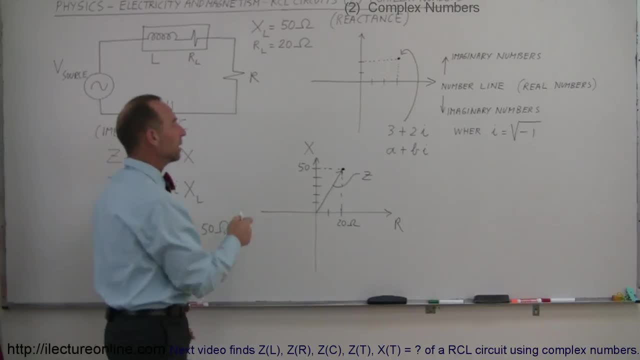 Alright, And that's how we look at impedance and that's how we indicate that. Now notice that it will have what we call a phase angle. That impedance has a phase angle. it's this angle right here, theta, and, of course, if you want to find that phase angle, 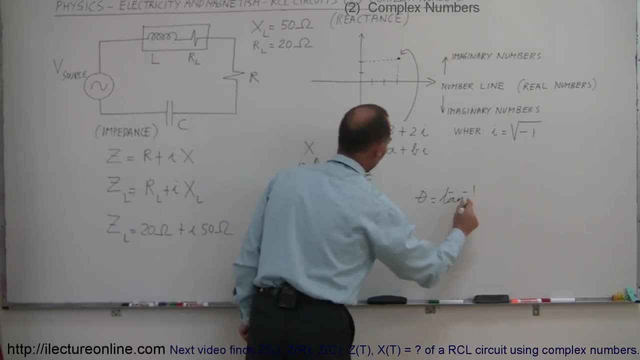 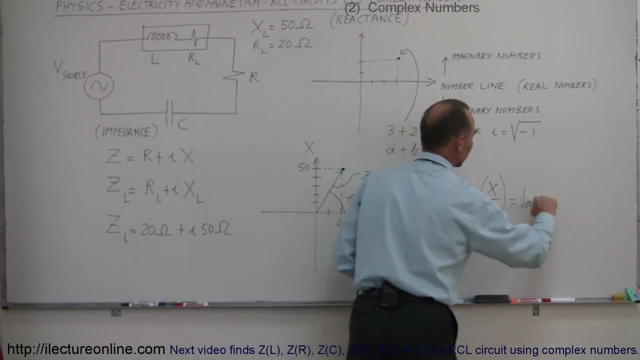 the phase angle, theta is equal to the arc tangent of the opposite side, which would be the imaginary part, that would be X divided by the horizontal side, which is the real part, R. So in this case the phase angle would be the arc tangent. 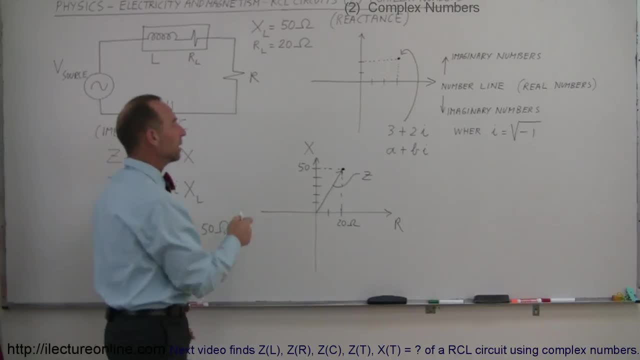 Alright, And that's how we look at impedance and that's how we indicate that. Now notice that it will have what we call a phase angle. That impedance has a phase angle. it's this angle right here, theta, and, of course, if you want to find that phase angle, 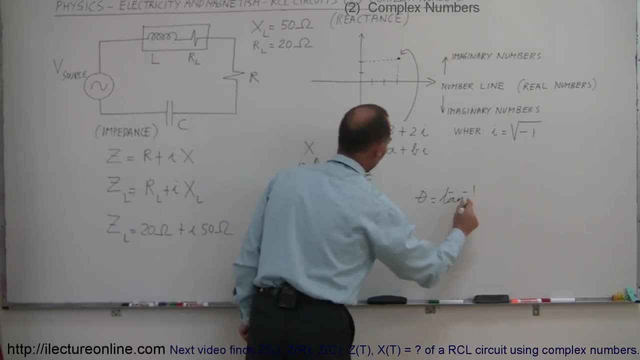 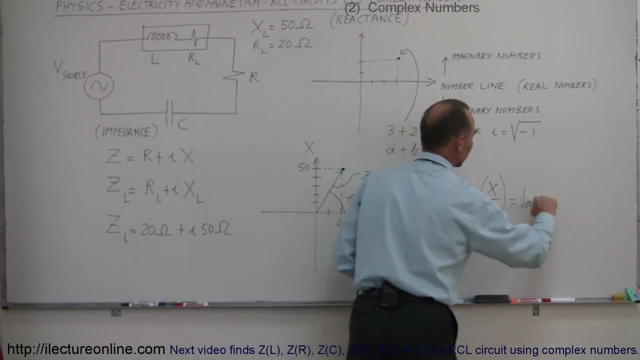 the phase angle, theta is equal to the arc tangent of the opposite side, which would be the imaginary part, that would be X divided by the horizontal side, which is the real part, R. So in this case the phase angle would be the arc tangent.